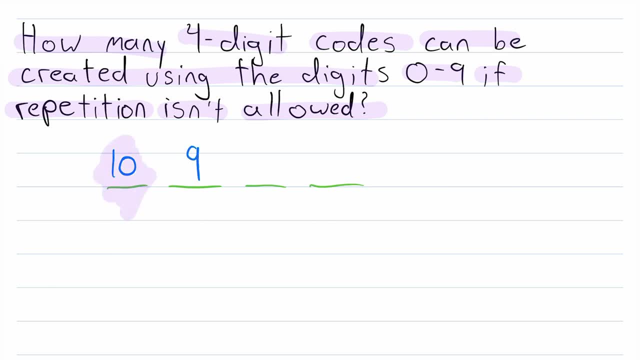 for every 9 options remaining, So for every 10 digits that could go first, there are 9 digits that could go second, which means we're multiplying these numbers together, And then this pattern continues. There are 8 digits that could go third and 7 digits that could go last, And again. 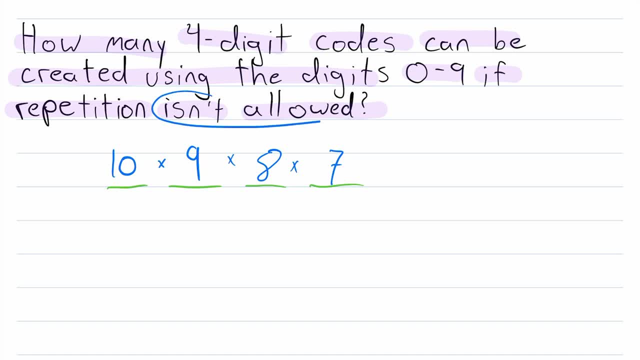 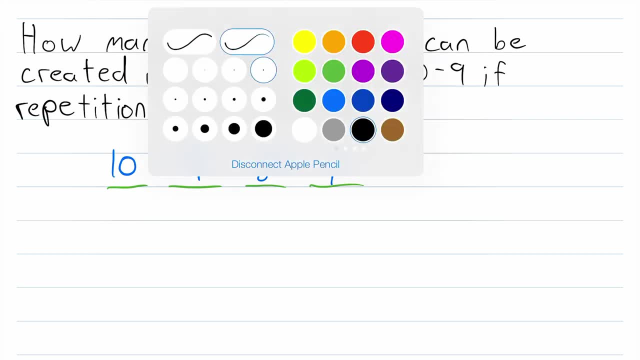 the number of options is decreasing because repetition is not allowed. So, again, this is a very typical example of a permutation question where repetition isn't allowed. But let's make a change. What if we say that repetition is not allowed? Well, let's make a change. What if we 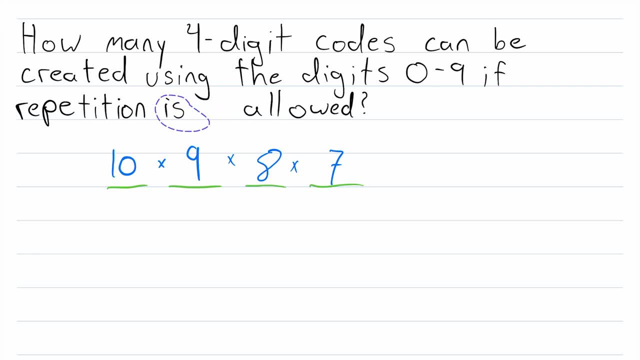 say that repetition is allowed, So now we'll be allowed to use the same digit multiple times. Then of course, there are still 10 options for the first digit. But now, whatever digit we use first, we can also use second. So instead of 9 options for the second digit, we still have 10. 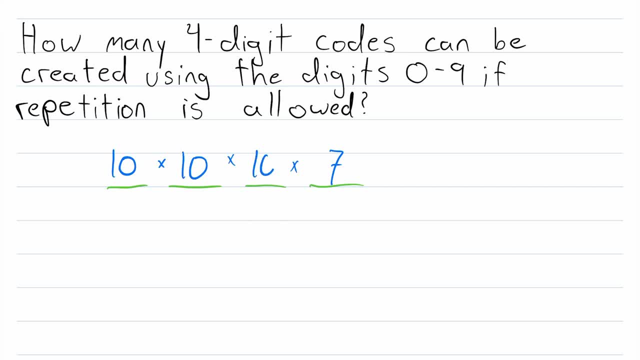 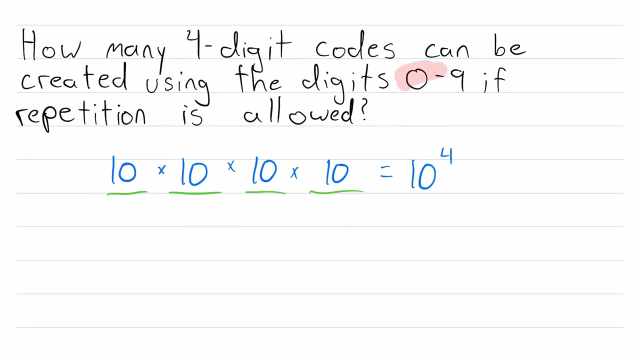 options. Same for the third digit: We still have all 10 options. And for the fourth digit, again, we've got all 10 options. So in this case there are a total of 10 to the power of 4 possibilities. So problems where repetition is allowed are very simple. We have: 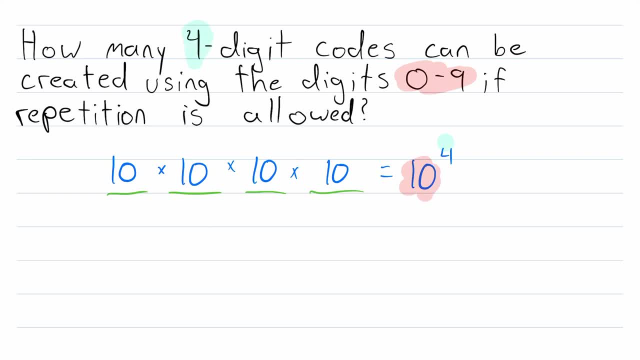 10 objects to choose from and we are ordering 4 of them. The total number of possibilities is the collection size to the power of the number of objects. we're ordering 10 to the power of 4.. I also want to point out, to prevent any potential confusion, another type of permutation problem. 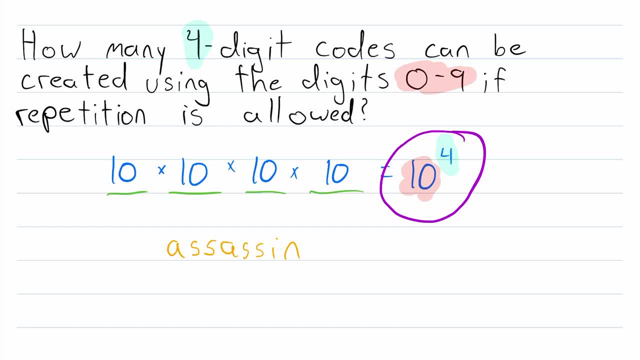 you might see, is a problem asking you: how many ways can you rearrange the letters in some word that has duplicates of one or more letters? I just want to make clear that this is a different type of problem that requires a different solution, But there are videos with similar titles to this one that are actually 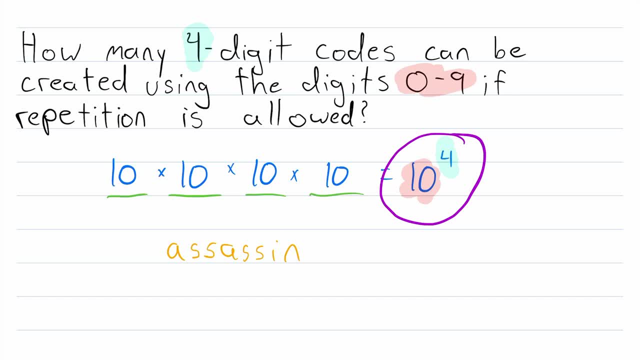 talking about this sort of problem. You can see, the key difference between these problems is that in this problem, repetition is allowed. We can use any of our 10 objects as many times as we want. So we can use any of our 10 objects as many times as we want. So we can use any of our. 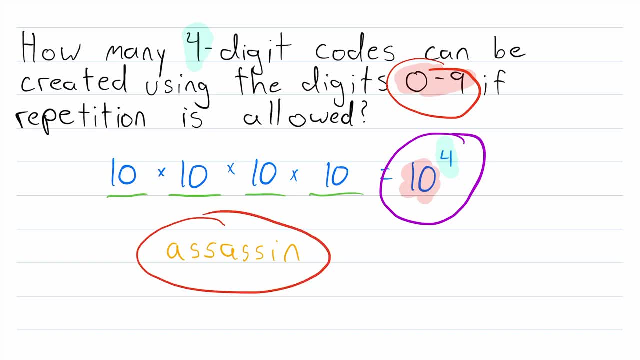 10 objects as many times as we want, Whereas in this problem some repetition is allowed, but it's a lot more particular. For example, we can use A multiple times, but it needs to be used exactly twice. We can use S multiple times, but it needs to be used exactly four times. I and N both have 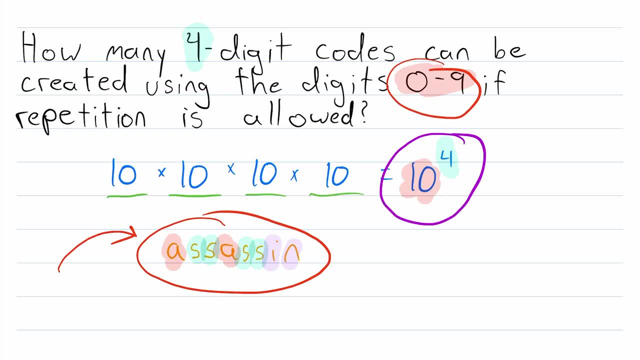 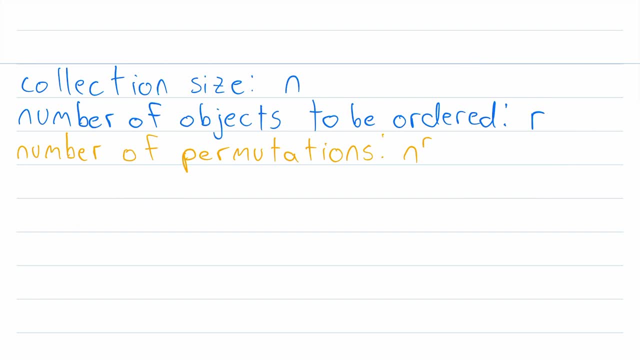 to be used just once. So this is definitely a different and trickier type of problem And, with that said, here's just a nicer description of the property we went over a minute ago. If we have a collection of size N and we are ordering R objects from that collection, 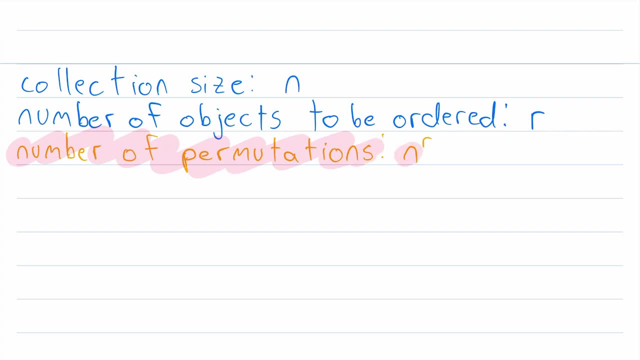 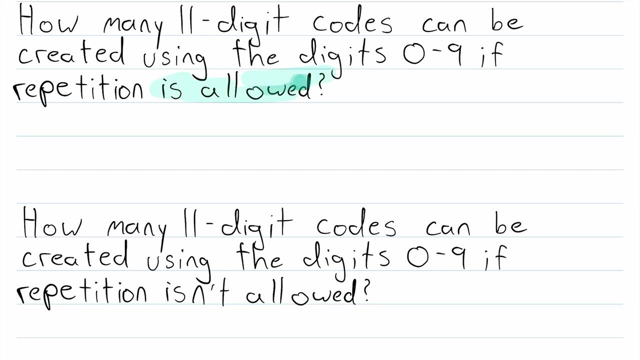 then the total number of permutations possible is N to the power of R, That's the collection size to the power of the number of objects that are being ordered. And then here's one last example to demonstrate how important the distinction is between repetition being allowed or not being. 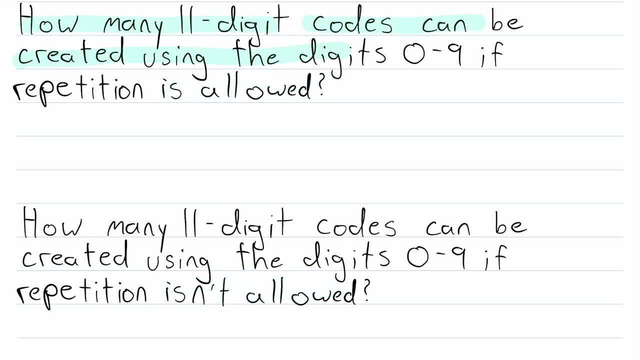 allowed. How many 11-digit codes can be created using the digits 0 through 9, if repetition is allowed? Well, the size of our collection is 10.. There are 10 digits to choose from And we are ordering 11 objects because we're counting the number of 11-digit. 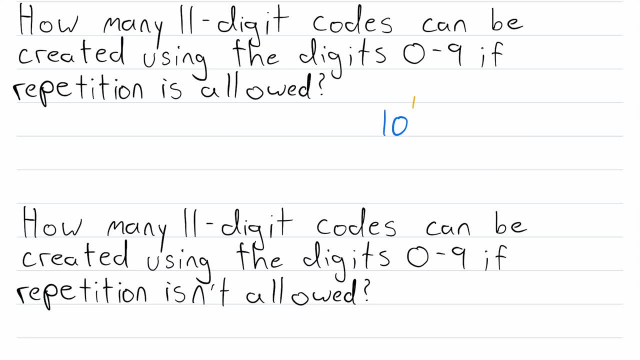 codes. So the total number of possibilities is 10 to the power of 11.. We've got 11 spots and 10 choices for all of them. Now here's a similar question: How many 11-digit codes can be created using the digits 0 through 9, if repetition isn't allowed? 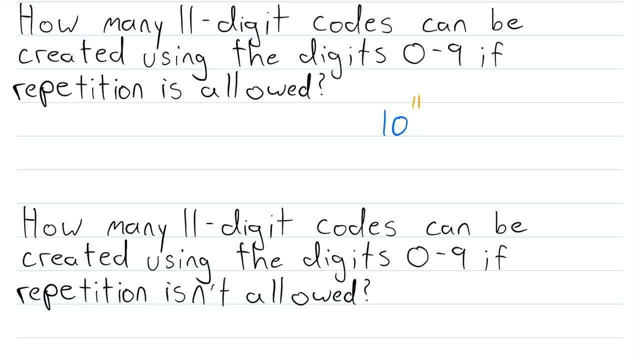 So think about that for a minute. How many 11-digit codes can be created using the 10 digits 0 through 9? where repetition is not allowed, It is of course 0.. We can't create any 11-digit codes with 10 digits if repetition isn't allowed, because, of course, 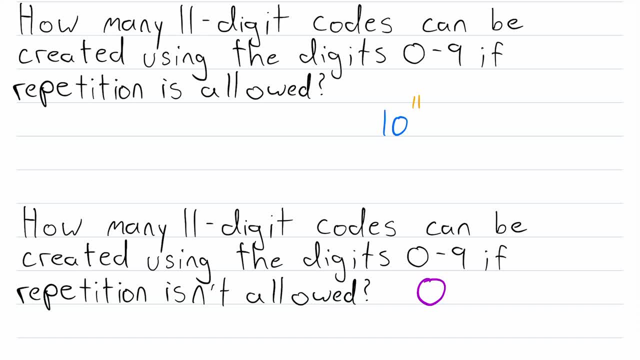 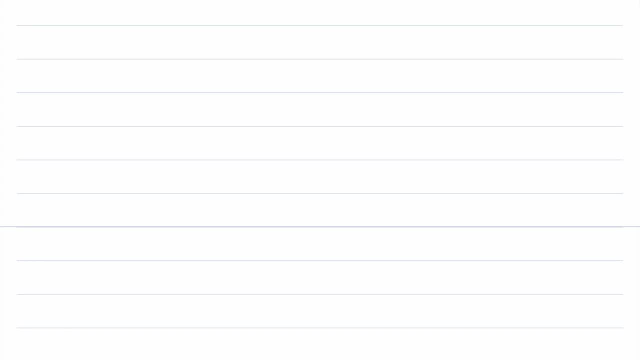 10 is less than 11.. So we simply wouldn't have enough digits to make a code, And that is a very big difference. Now let me just leave you with an example to try on your own. How many 7-letter passwords can be created using a 26-letter alphabet, if repetition is allowed? 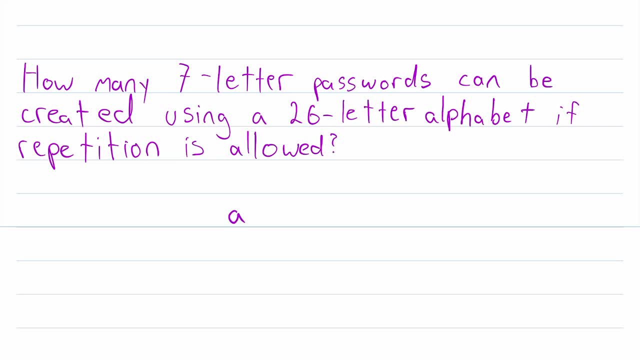 And, for the sake of this problem, assume that the case of the letters doesn't matter. So, uppercase or lowercase, that does not matter. There are 26 letters to choose from. Let me know what you get down in the comments and I'll leave the solution in the description. 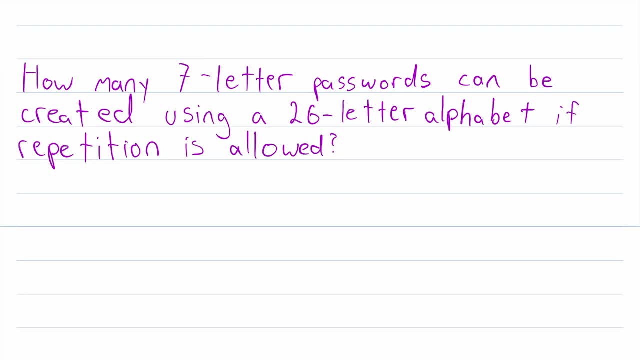 So I hope this video helped you understand permutations with repetition. Let me know in the comments if you have any questions, need anything clarified or have any other video requests. Thank you very much for watching. I'll see you next time and be sure to subscribe for the swankiest math lessons on the internet.